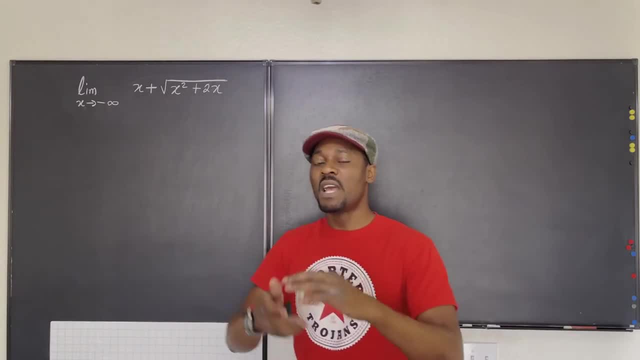 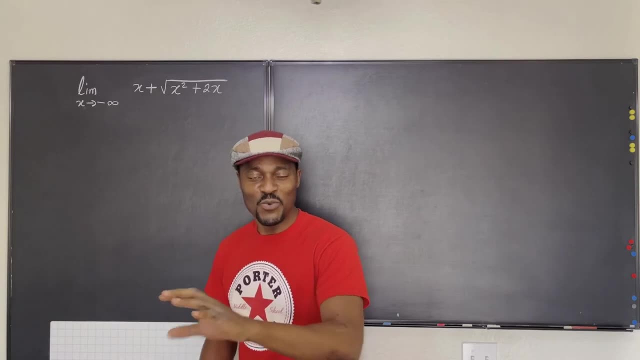 or subtracting infinities or things approaching infinity. You want to express your term or your expression in terms of rational expressions? Okay, you want to create fractions, because with fractions you can know what's going to happen as x goes to infinity. But if you don't have fractions, it's a little bit difficult to decide. 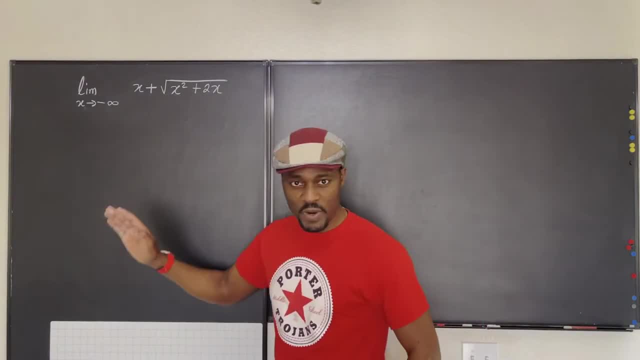 what to do or what your output is going to be. So what do you do in this case? Always do this: You want to rationalize this expression. Now, when I say rationalize, it means you want to give yourself something that gives you a reasonable rational expression. that is fraction, So multiply. 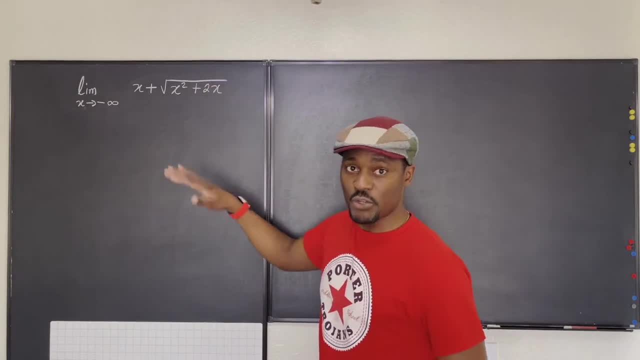 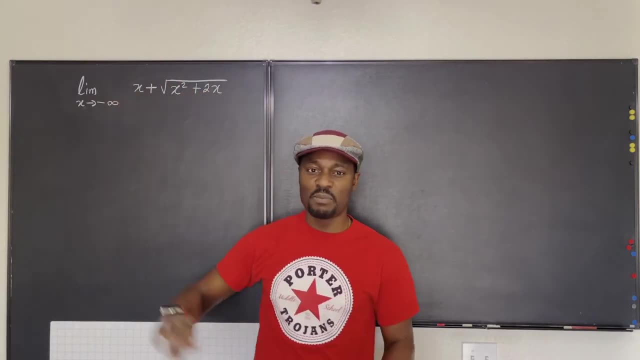 this by its conjugate and also divide it by its conjugate, so you don't change the value of what you have. So I'm going to do the work on this side and then we come back here and continue with the limit. But how can we change this expression to make it usable? So what we're going to say is: 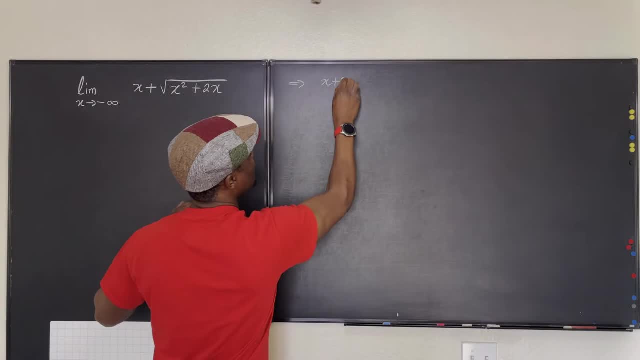 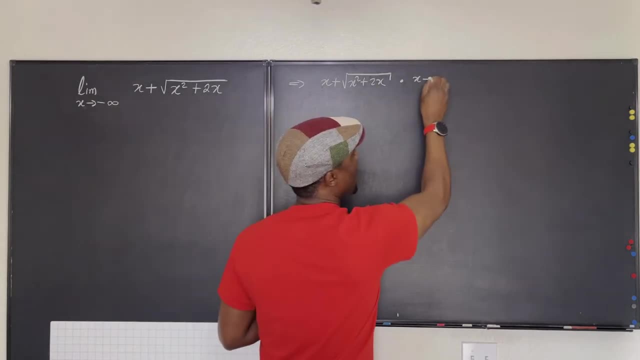 that we're going to multiply x plus radical x squared plus 2x. We're going to multiply it by x, Instead of saying plus. now we just say minus, and that's the only difference: Minus x squared plus 2x. We do the same thing here. We divide it by x minus radical x squared plus 2x. You see, 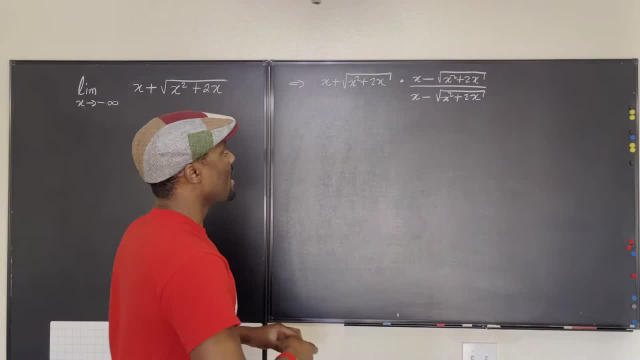 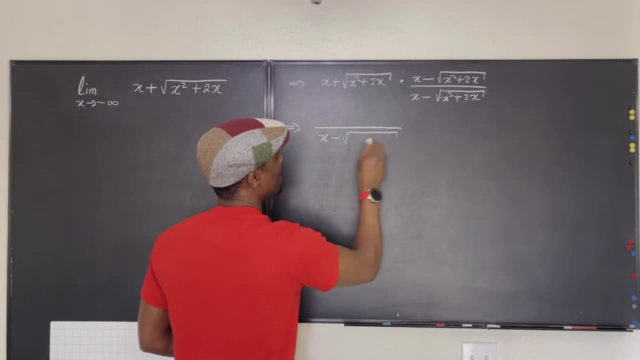 now we're going to have something that we can work with. So the next thing is to multiply the top. Well, the denominator is going to look like this, Just this: It's going to be x minus the square root of x, squared plus 2x, And then the top is going to be the product of this and this. Let's. 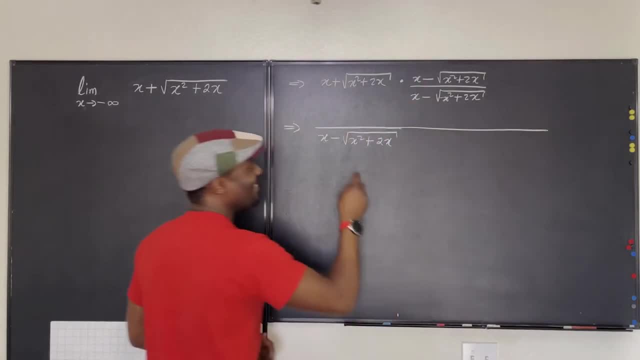 multiply that out. I think it's going to be a long expression. Okay, Well, this is going to be down here. But x times x is going to be plus x, squared plus 2x, And then you multiply it like this: So: 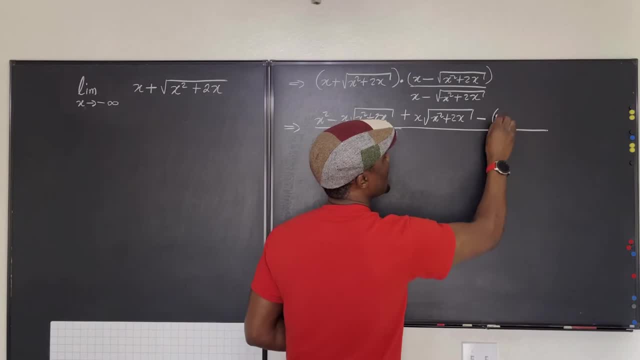 you're going to multiply this expression by this expression. Okay, So what I'm going to do is this is going to be just minus the square root of x, squared plus 2x, And this is going to be plus x squared minus x squared plus 2x. So that's the. that's what we have Now. we just need to simplify what's. 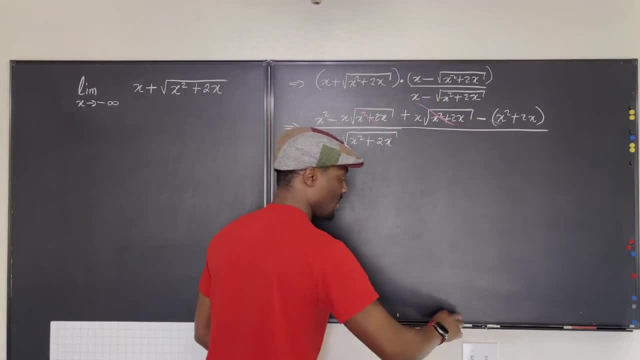 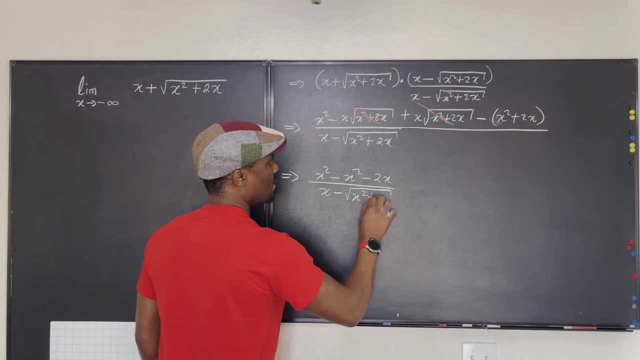 on top And we can see that this is the same as this, but just opposite side. So they cancel out And what we have left will be this expression, which is x squared. We open this up: Minus x, squared minus 2x, And this is going to be x minus the square root of x squared plus 2x. Well, 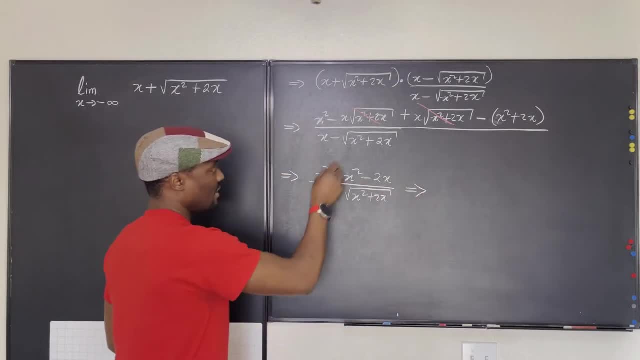 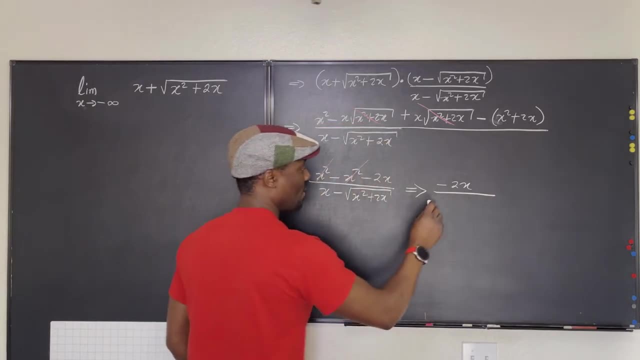 this is going to become. this takes this out again. This takes this out. Then we have negative 2x over what we had before: x minus the square root of x, squared plus 2x. Now I want you to see as a general thing that you will always have the opposite side of this in. 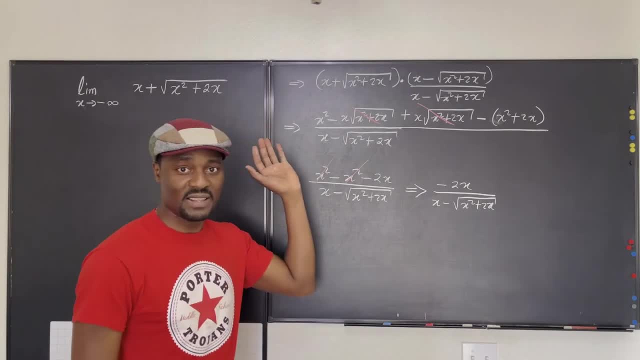 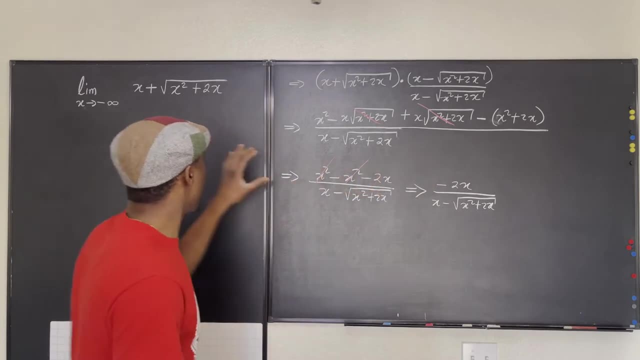 the denominator And that's all you're going to have, unless the question is more complicated than this. But if it's in this form, you'll always have that in the denominator. Okay, Now, what can we do? We need to take this now and write it back here, because that's the limit we're about. 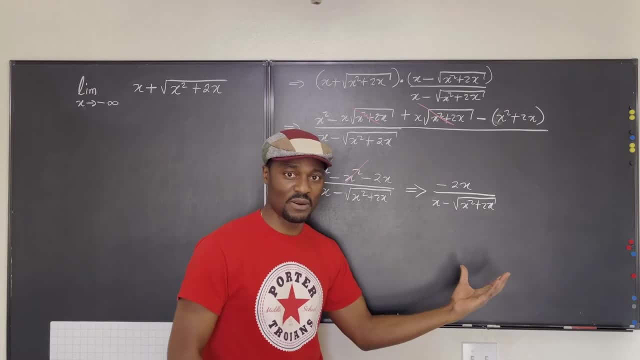 to take. Now, you see, we're not subtracting any two terms. We have a single term, The numerator and the denominator, And that's easier to work with when you're dealing with infinity or negative infinity. Okay, So let's rewrite the question. So we have the limit. 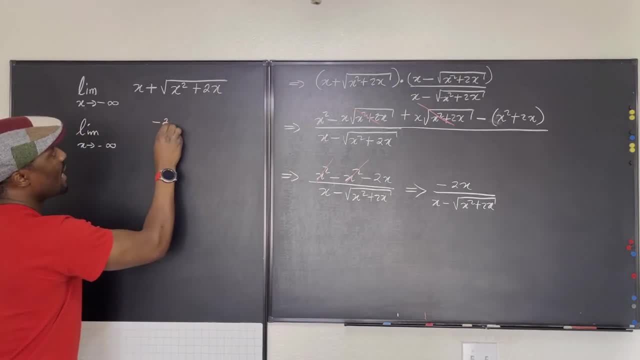 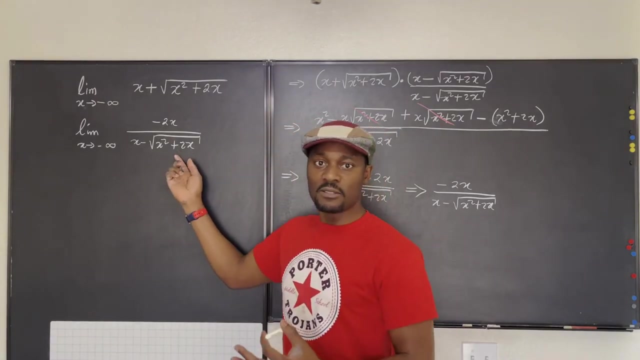 as x goes to negative. infinity of negative, 2x over x minus radical x squared plus 2x. So what you have here, what are you going to do? Remember, whenever you have a rational expression that contains a radical term, okay, or? 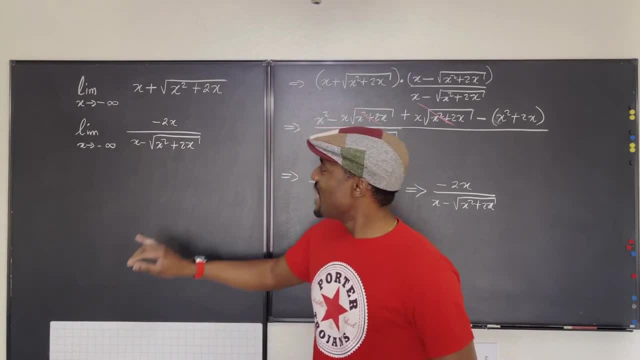 what you call radical term, and then it goes to infinity. what you want to do is divide both the top and the bottom by the term in the denominator that has the highest exponent of x. Well, based on what we see, this is the highest exponent: It's 1, because it's not x squared. 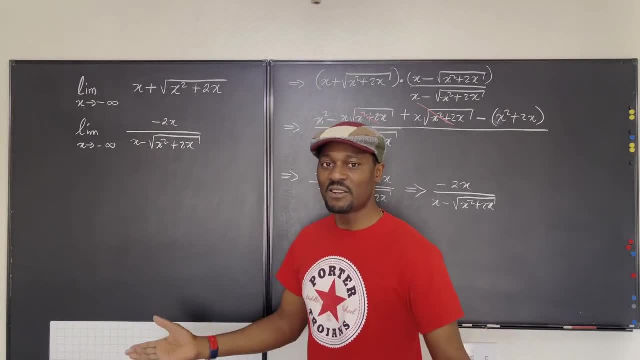 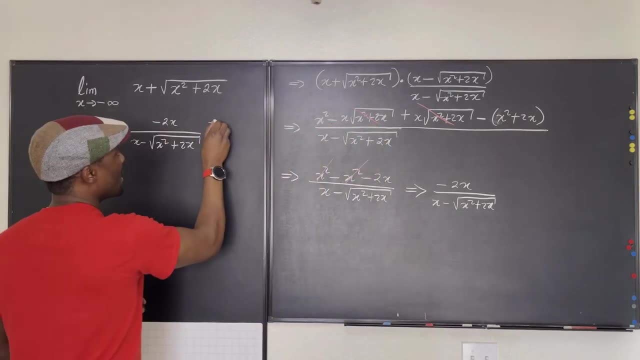 because the square root of x squared will still be x to the first. So that's the highest term that you can deal with And that's what we're going to do. We're going to divide both the top and the bottom by this term. Okay, So we're going to say: divide by x, divide by x. Well, 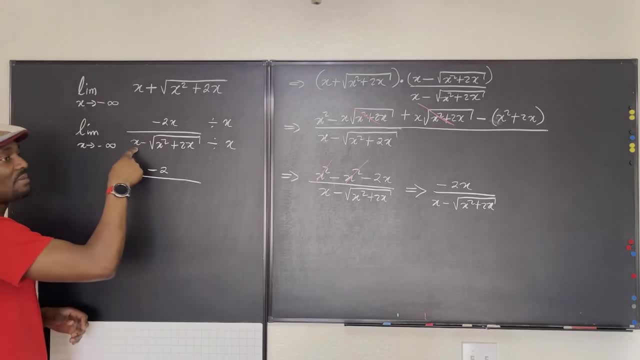 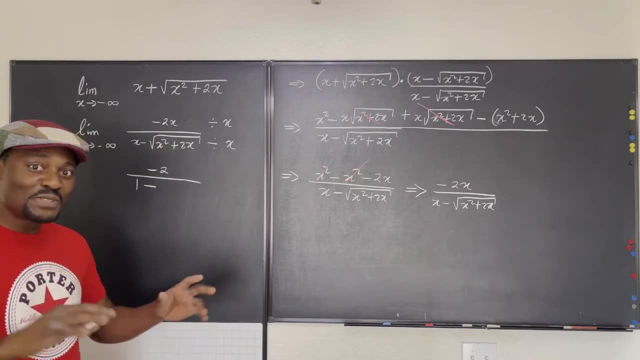 by x, you're going to end up with negative 2.. If you divide the bottom by x, you're going to end up with 1 minus. If you divide this by x, that's going to be something you've seen in my other video. What do you do? How do you divide something under the square root? 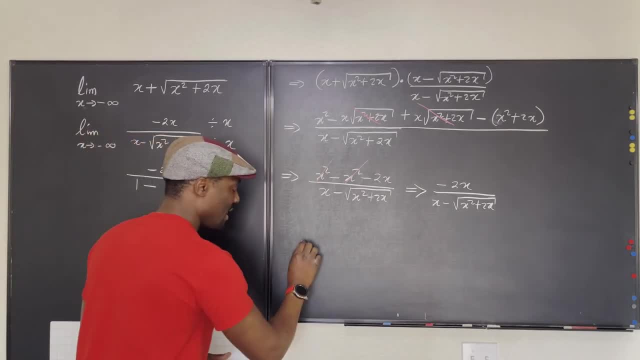 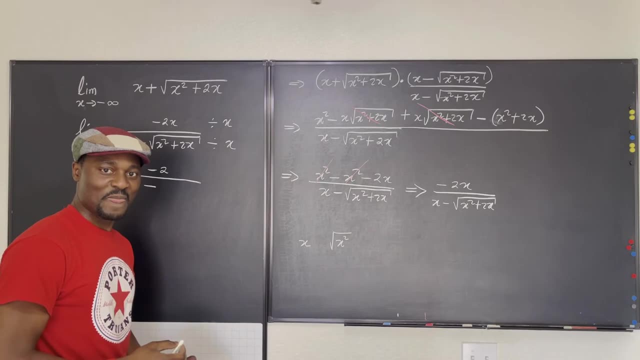 sign by what does not have a square root sign. Well, remember that instead of you writing x, you could as well write the square root of x squared. Do you see that? Okay, So instead of writing this so, we're going to push in x squared here. but there's something. 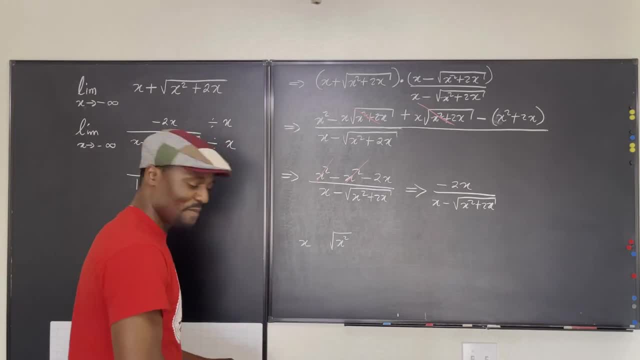 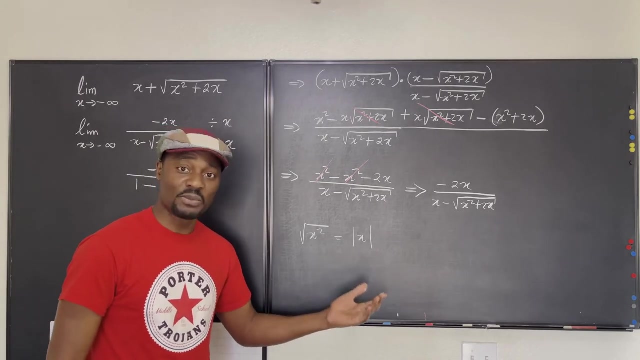 special about taking the square root of x squared. If you watch my other video, let me explain this. Whenever you take the square root of x squared, your answer is the absolute value of x, because it's possible that x is positive and it's also positive. I also possible. 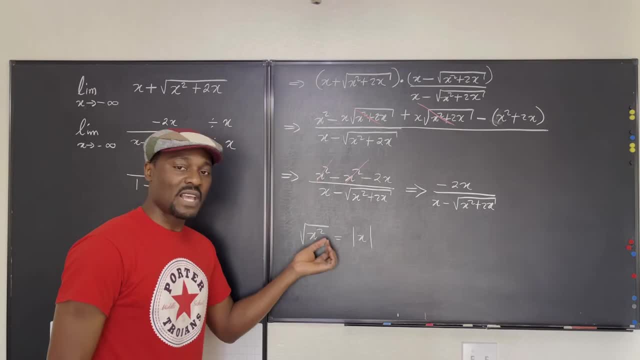 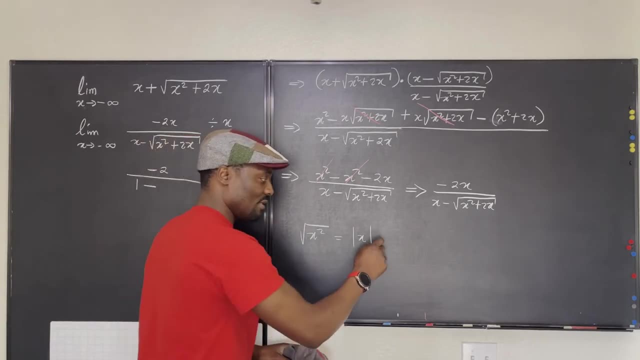 that x is negative, So you could have x x times x gives you x squared, or negative x times negative x gives you x squared, So you still get x squared. Now, when you take the square root, you'll have two options. Okay, This means you're going to have x squared. 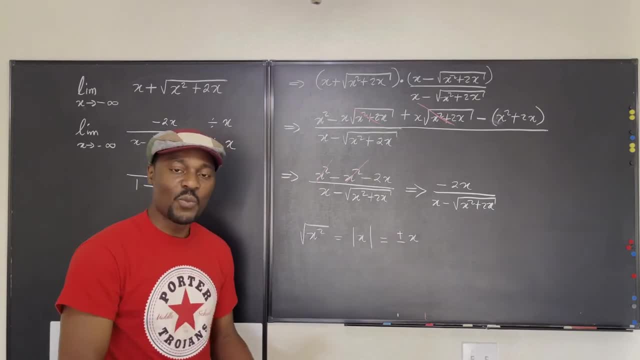 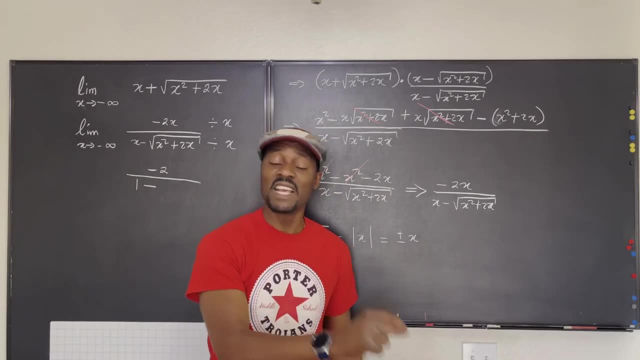 plus or minus x. Now, which option will we take? Well, that's where this is important. It says x is approaching negative infinity, which means we are certain that x is negative, but it's so negative it's approaching infinity. So the option you'll take in this case will: 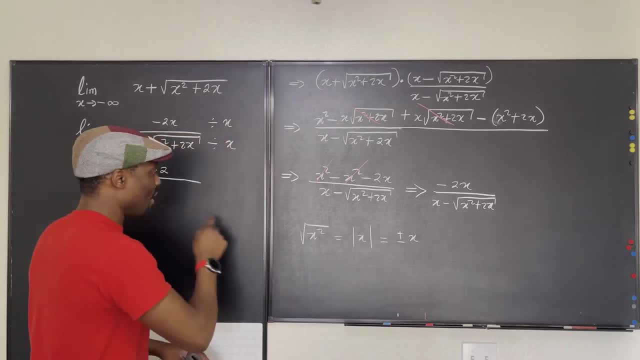 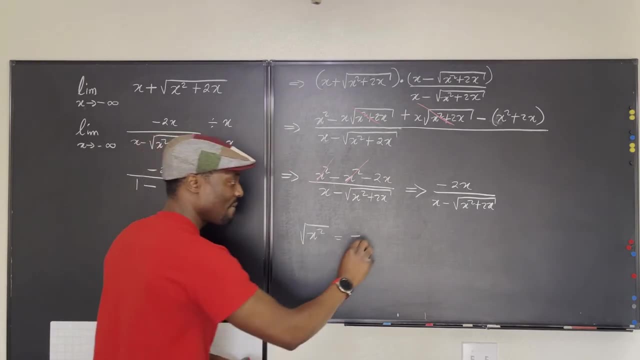 be the negative option. Okay, So therefore, when? so you can see that actually, the square root of x squared in this particular case is the negative of the square root of x squared, that would normally would take: Um, what are we doing? Well, this is the negative option because this is supposed to. 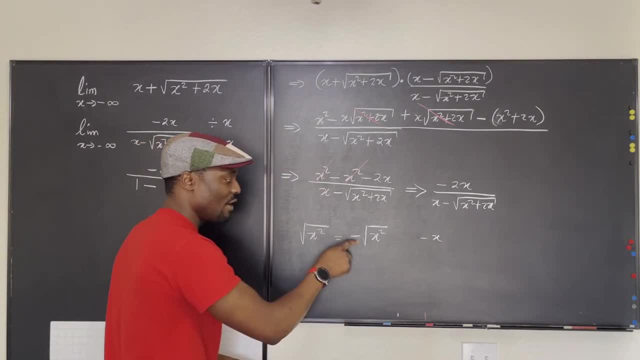 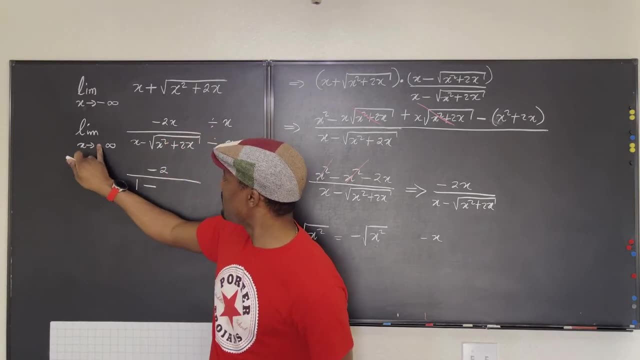 give you negative x. Okay, So you just put the negative sign here to show that you know you're going to get a negative answer because x is approaching negative infinity. If this was x is approaching infinity, your option would be the positive option and you wouldn't. 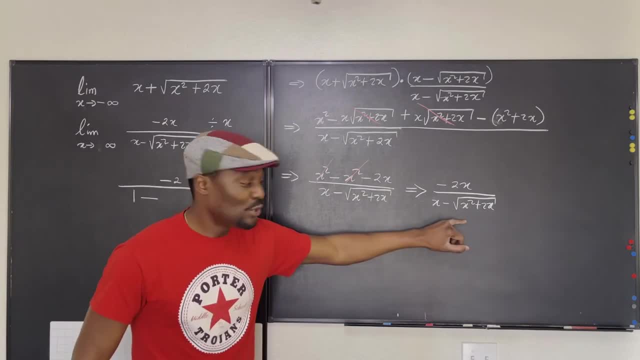 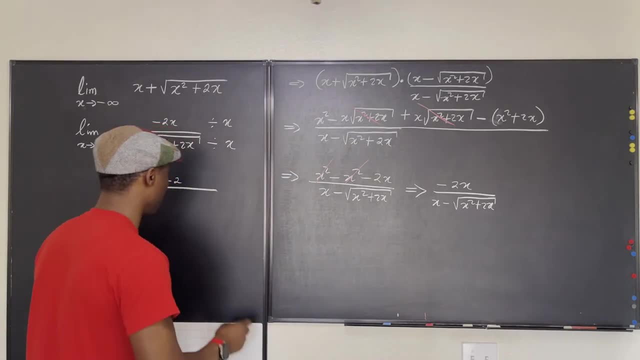 have to put the negative sign here, So I'm going to rewrite this point. So what I'm going to do here is, instead of writing x squared plus two x and then dividing it by x squared, based on that explanation, I'm going to say it's negative. 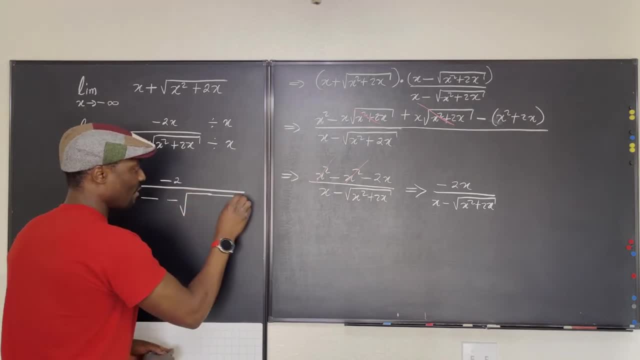 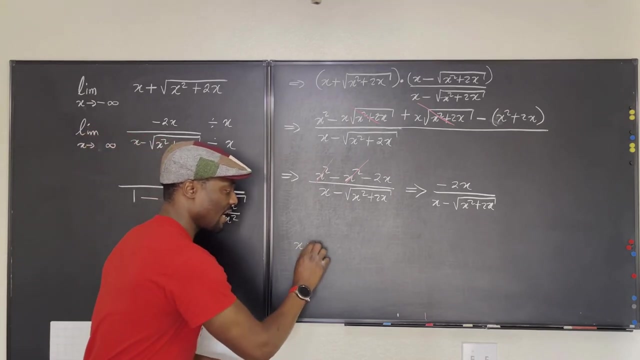 Okay, It's going to be negative. This is now going to be x squared plus two x divided by x squared, divided by x squared. See, this is the part that you need to understand. So why did I put an x squared here? Remember, I told you that x is the same thing as the? 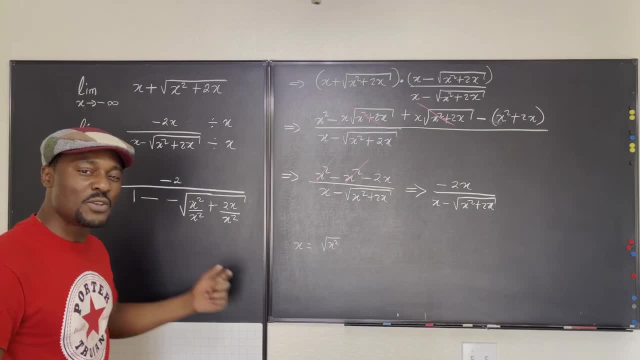 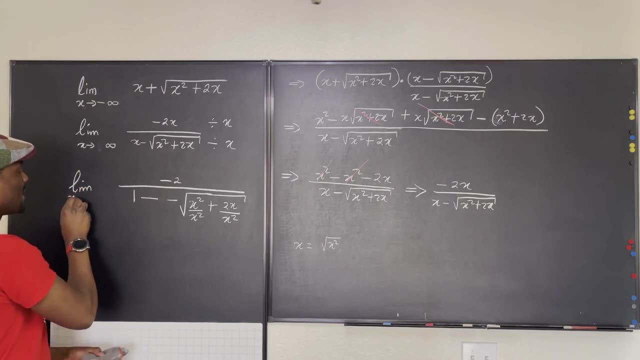 square root of x squared. Okay, But this x squared that is inside already. when you take the square root of it, it will be the negative option, So that's why we're going to have this here. So at the end of the day, we have the limit as x goes to negative. So we're 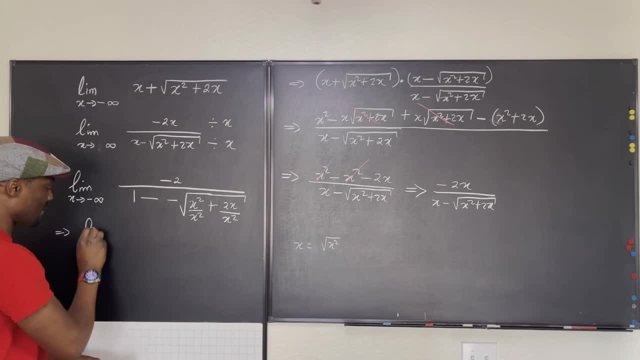 going to have negative infinity. So this gives us the limit, as x goes to negative infinity, of you have negative two on top, one here, minus Here. you're going to have minus again. You see that. So this is going to be a plus. So I'm just going to change this into a plus.